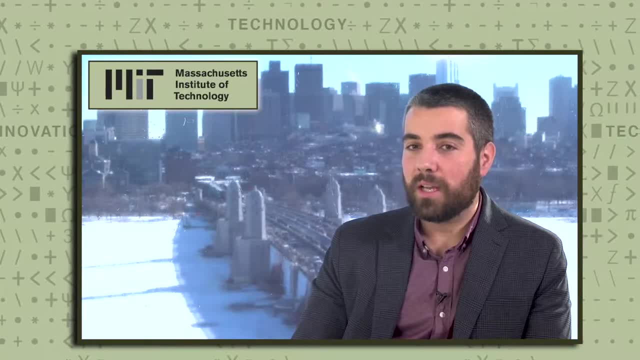 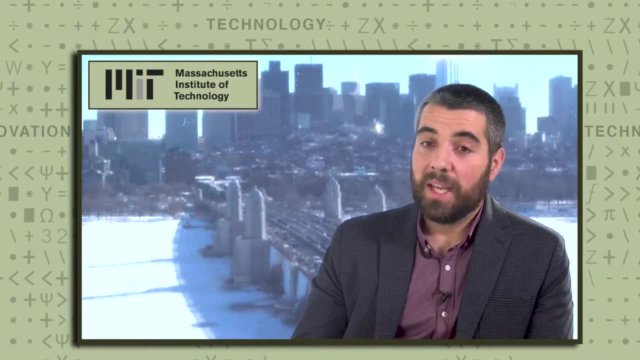 It's just a very complex process that involves many, many questions that, most of which we don't know how to answer yet One of them has been to show that we can recover some of that dexterity even if we use the kind of simple grippers that 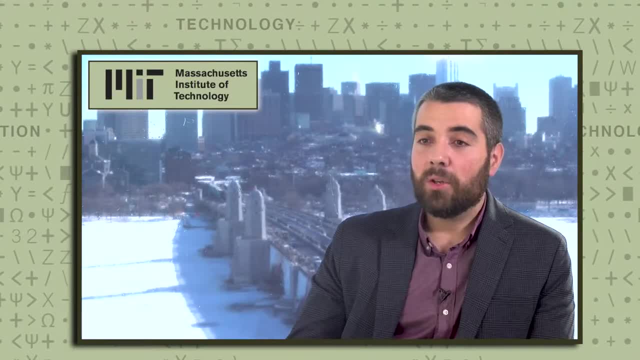 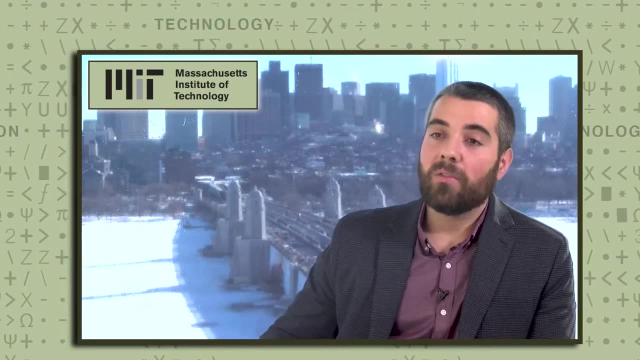 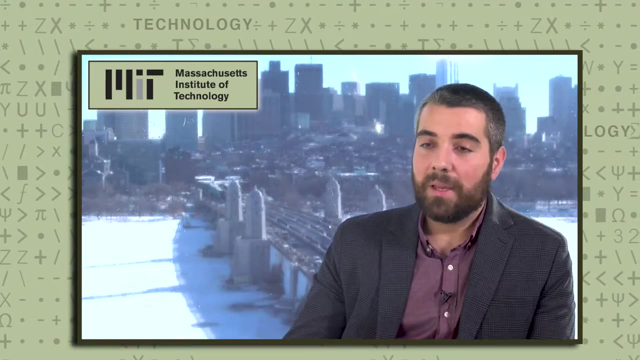 industry is used to use like parallel gripers by exploiting the environment. So similar to the way we grab a phone from our pocket and then flip it like using a dynamic motion or using gravity, or just tapping a pen on a surface to be. 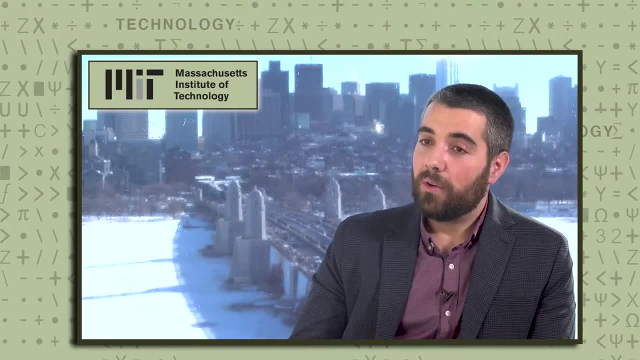 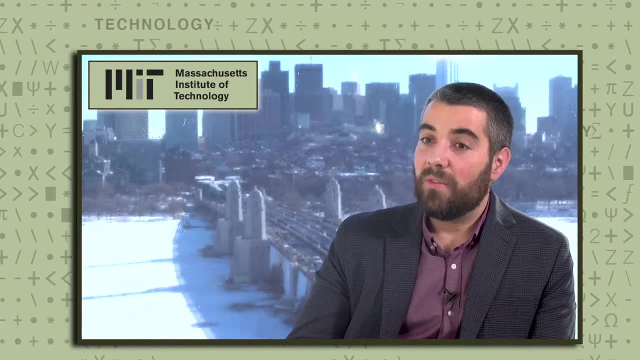 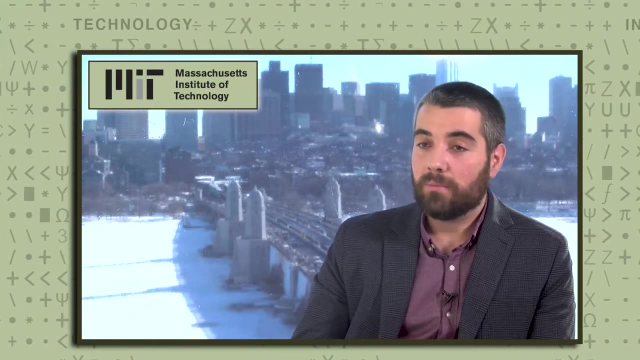 able to get the right grasp. We've sort of been working for some time now on automating the process of the robot thinking or figuring out how to use the environment to manipulate objects, So that even robots with simple grippers, like the ones that we find today in industry, can't manipulate parts without 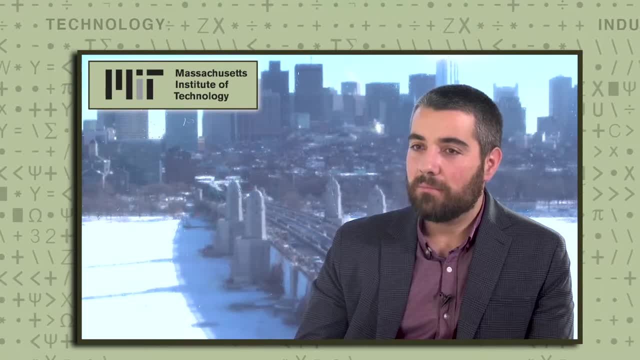 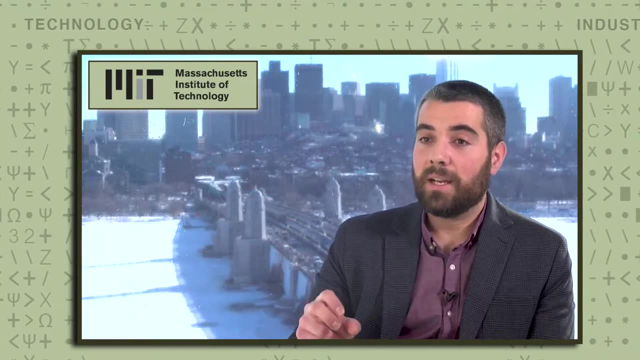 needing to have like a very expensive and complex hand, like a human hand. Yeah, so the robot is presented with a part, it picks it up and then it's just a parallel gripper, so there's not much that it can do with it. if we're just looking at. 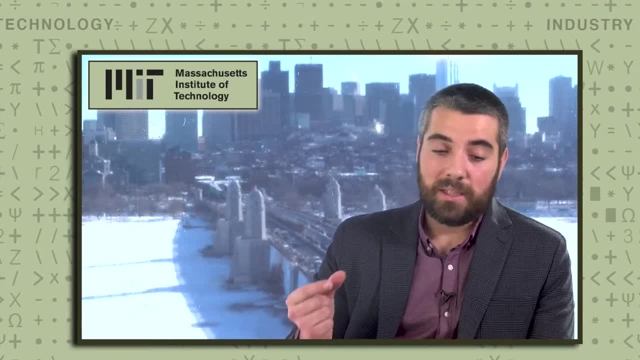 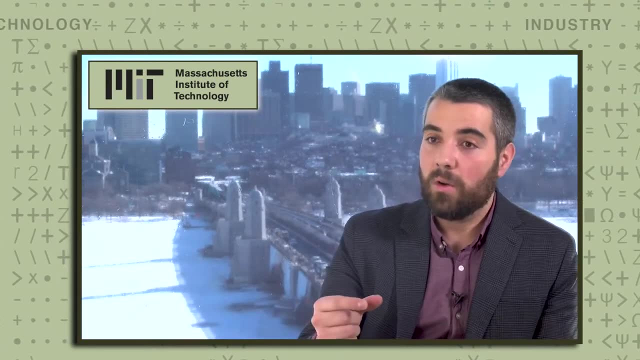 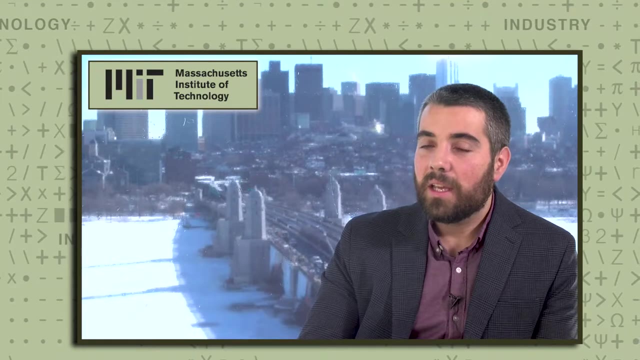 the gripper itself, But now it needs a different grasp. so what it does is it goes against the floor and then uses the floor as an extra finger, or it goes against a wall or against a fixture design as an extra finger So it can change the grip on the object without having to put the 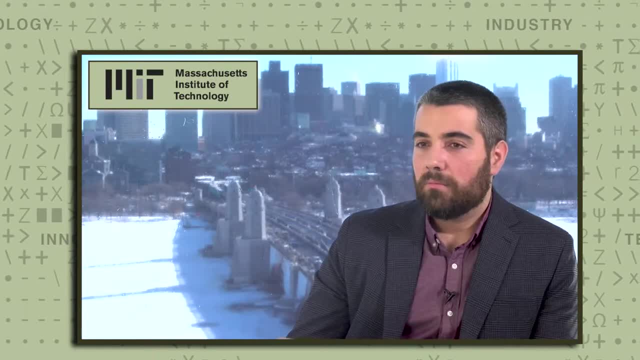 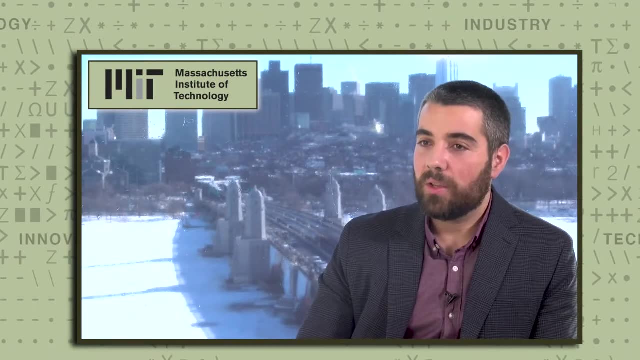 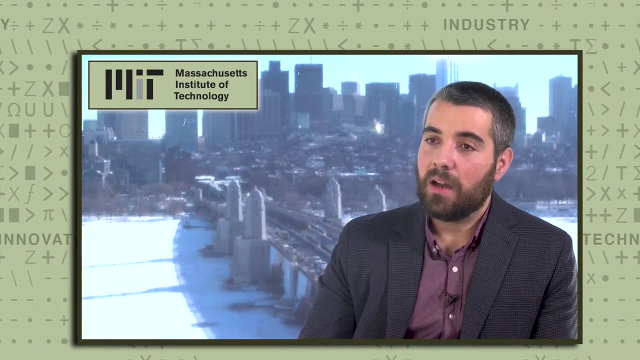 object down and pick it up again, which for industry, that just means more like productivity, efficiency, right, It allows the robot to go faster to the things that it wasn't able to do before. You need to give the robot a sufficient understanding of the mechanics of physical 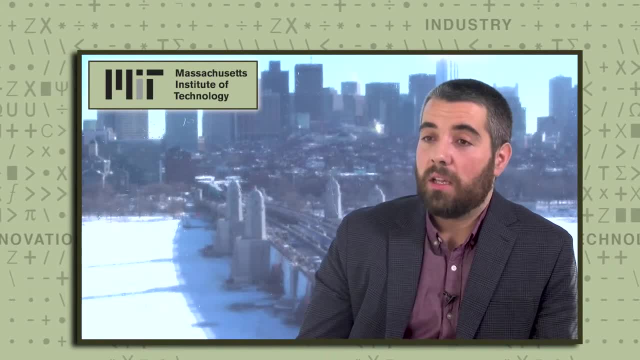 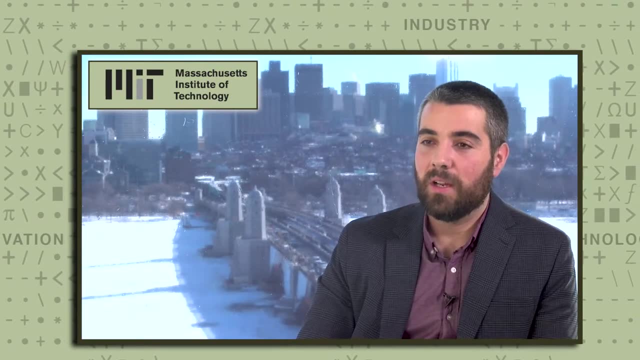 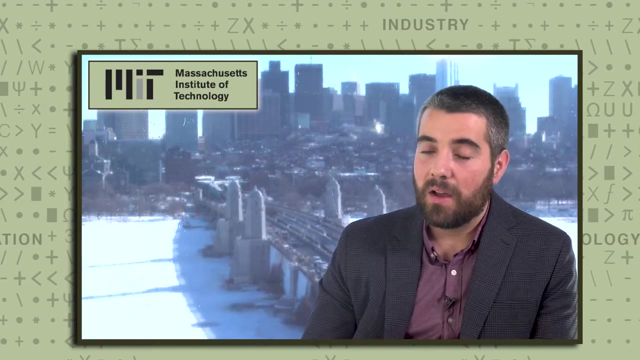 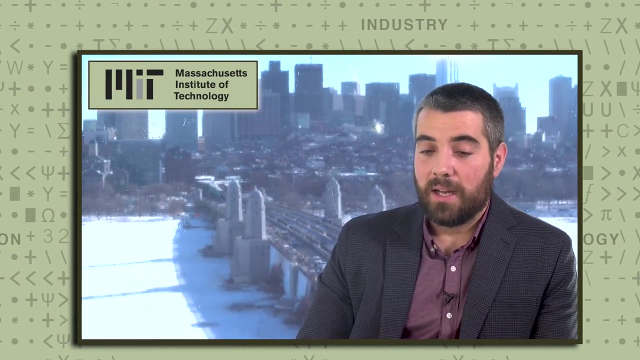 interaction, which is an understanding that we've had right. Physics is something that the physics of contact interaction has been known for for a very long time, but boiling it down to a set of equations that are simple enough that the robot can exploit explicitly is something that it has been difficult to do, And we've sort of figured.